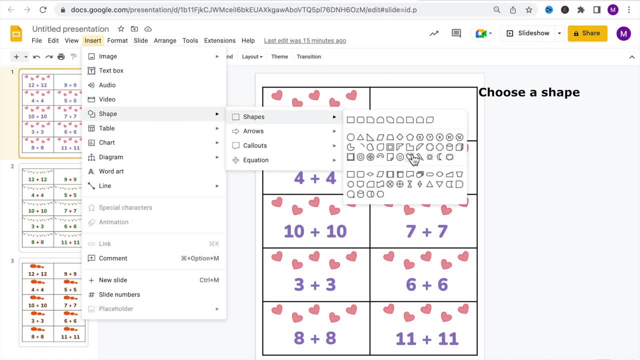 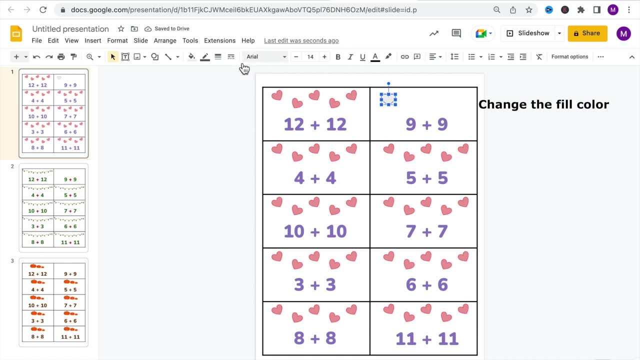 onto your resource. Here I'm going to choose a heart. Once that loads up, I'm going to change the colors. I'm going to choose a lighter red to fill in the heart and for the outline I want a darker red. Next, you can play around with how that shape is presented. I'm going to adjust the. 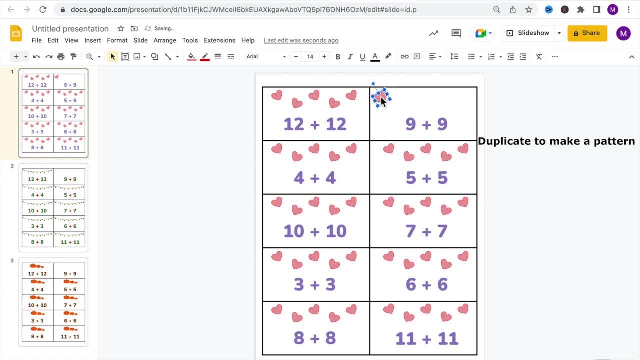 rotation of the shape and duplicate it to make a fun pattern. To duplicate any shape or item on your keyboard, press command d or control d. I want five of the hearts and I want them across the top of each heart. I'm going to add a heart to each heart. I'm going to add a heart to each heart. 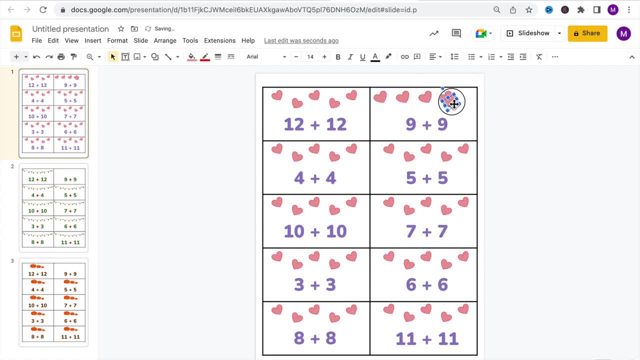 And remember, you're going to cut these out, so think about that when you're spacing out your clip art or shape. Last, I'm going to move around the rotation of every other heart and then move every other heart down just a bit. Something else that I did was change the color font of the text. 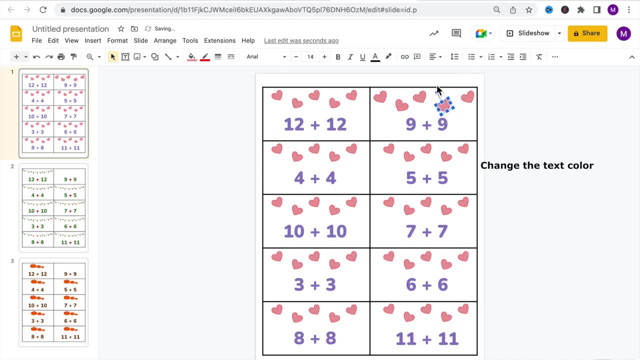 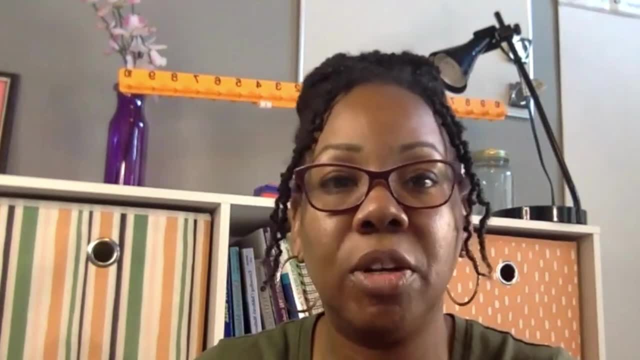 so I have the red for the hearts and purple for the text. Do this for the resources that you repeat each week or each month, such as for centers, stations, individual events and so on. If you have any questions or comments, feel free to reach out to me. 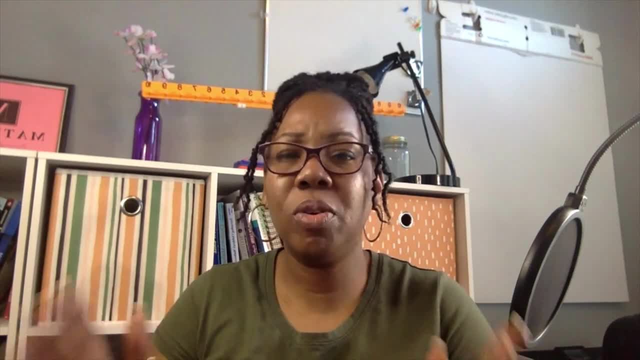 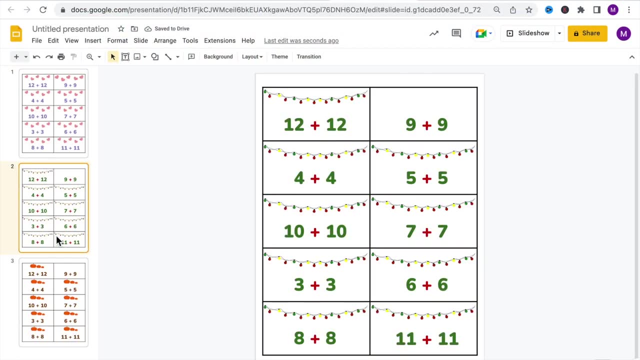 If you don't have a color printer, you can still use the shapes. just don't use a fill color or use black or gray. Another popular holiday to create your math resources for is around Christmas time. You can use another shape or you can find a fun piece of clip art, such as a present. 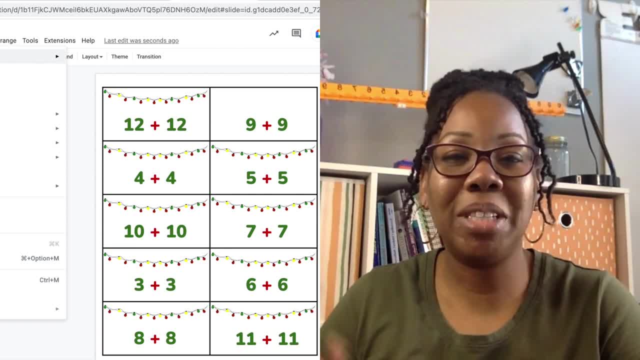 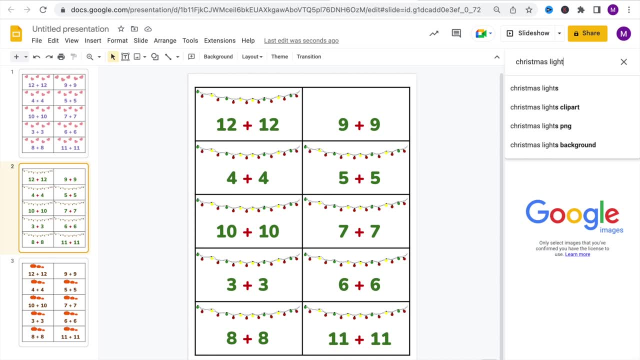 ornament- a Christmas tree or a small snowman- I thought about using Christmas lights. so after going to insert image, then search the web, I typed in Christmas lights clip art and had it in the library. I had a few different options come up. Find the one that you want, select it and scroll. 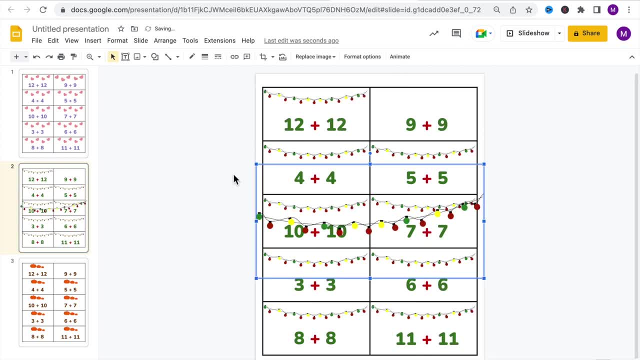 down to press insert and the image will pop up for you. Next, resize the image to fit whatever resource you're working on. Again, in my case, it's the flash cards. Make sure the image is brought to the front and then position it how you want it. Just like the hearts, I want my lights going across the top. 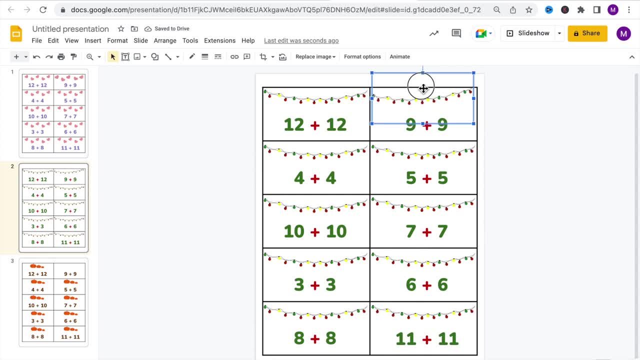 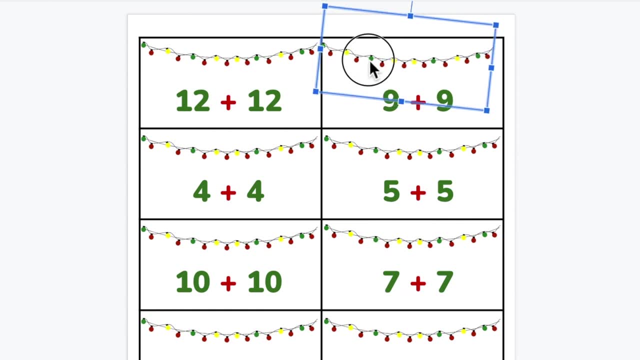 of the flash card, making sure it's not where anything will get cut off. Last is the color for the text. Here I have the text in two different colors. I'm going to use the color of the text in two different colors. The digits are in a green font and the plus sign is in red. Again, if you can't, 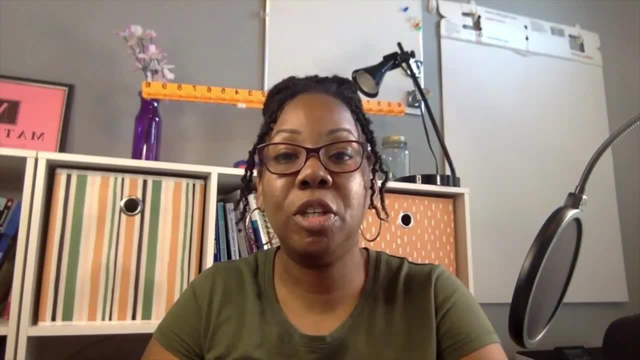 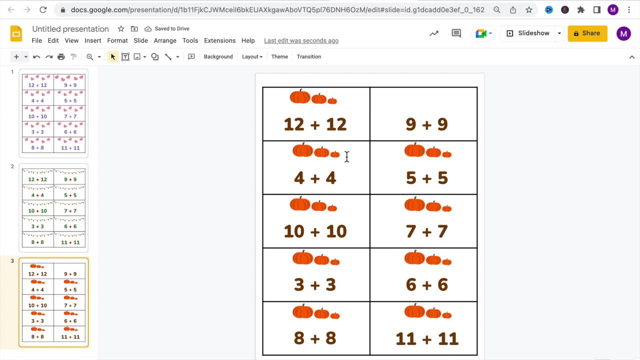 use color. keep it in black or shades of gray. Another option, using the clip art for a theme around October or November could be a harvest festival or something for Thanksgiving. I wanted to choose something like a pumpkin, so, again after going to insert in the ribbon, then image and search, 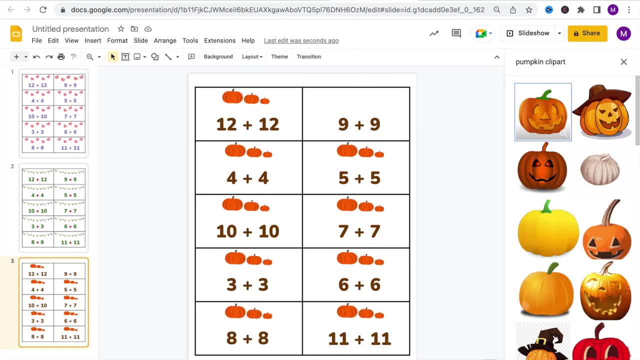 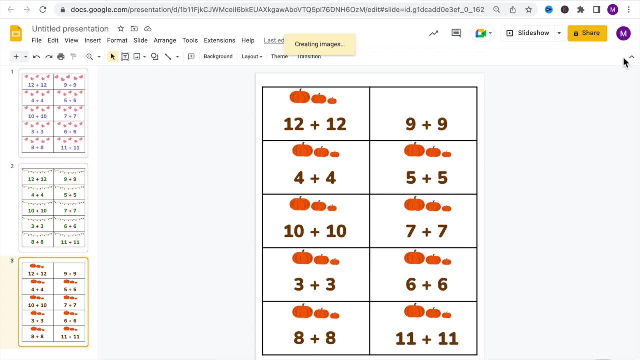 the web, I typed in pumpkin clip art. A lot of them were jack-o'-lanterns already, but I wanted just the pumpkin Again, once you find the image that you like, select it and click insert. This time I wanted to make a group. 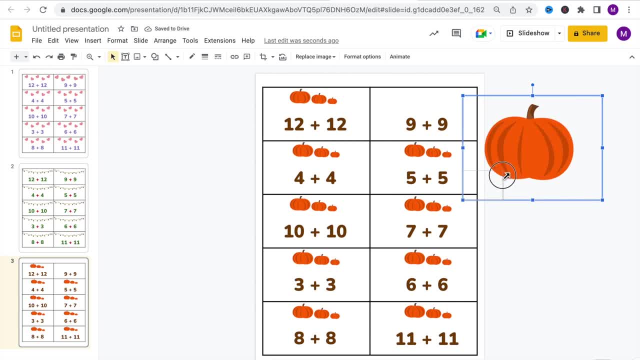 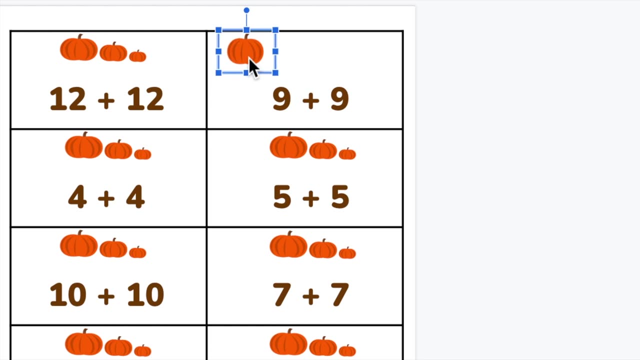 of images. I moved the pumpkin over to the side. I want three of them in different sizes. Remember to make sure they are all brought to the front before grouping them, and I probably should have grouped the hearts together in the first example, Seeing where I wanted that pumpkin to go next. I 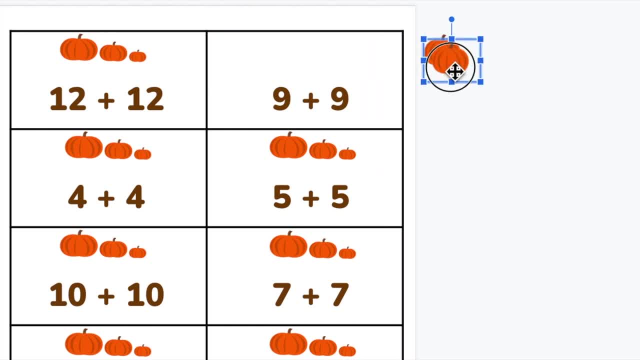 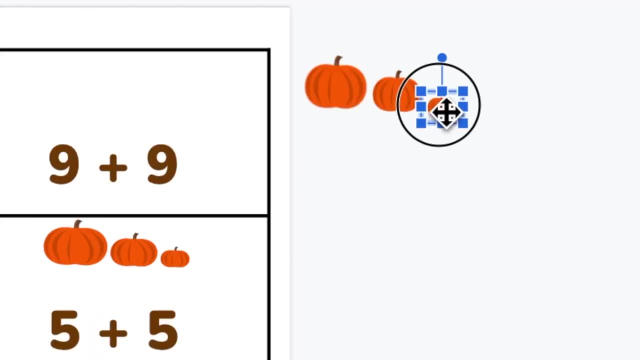 moved it back over to the side, hit command or control D to duplicate it, then decrease the size of the pumpkin and placed it closer to that first pumpkin. I hit command D again so that I could have a third pumpkin and decrease the size of that pumpkin as well Once you have your pieces of clip. 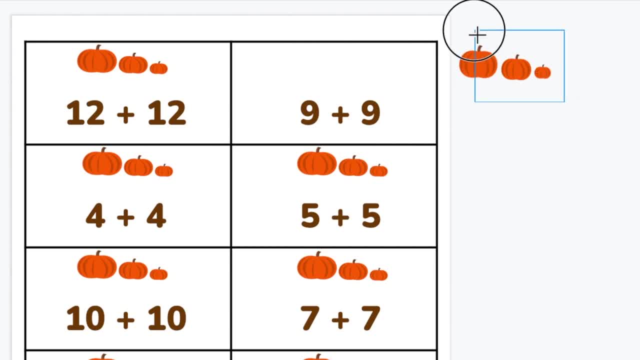 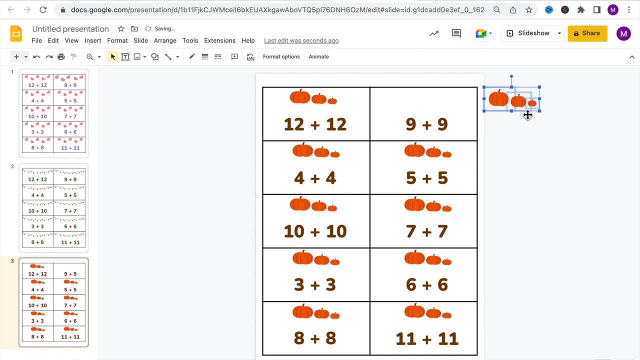 art where you want them together. select all three of them and right click while they are selected so that you can scroll down to select group. Now they will only move together in those same positions. Position the group where you want it. on your resource: Again, I wanted the theme at the top of the flashcards. Think about where you will put yours. 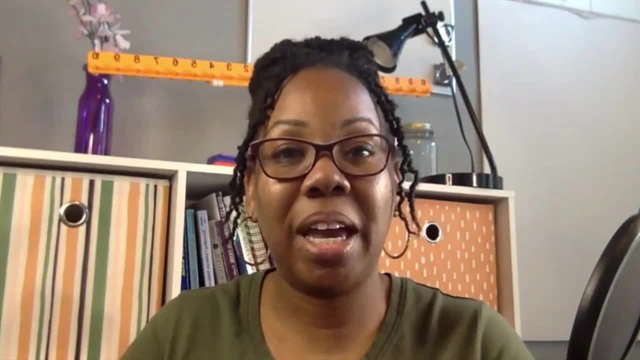 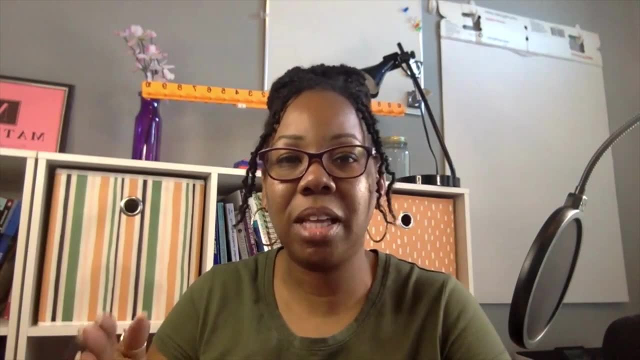 So that's how you can spice up the math resources you have already created or plan on creating with a fun theme for any holiday or season. But if you're saying, hey, how do I make flashcards like the ones you've been showing me in this video? Don't worry, I have a video for you to watch, right. here,